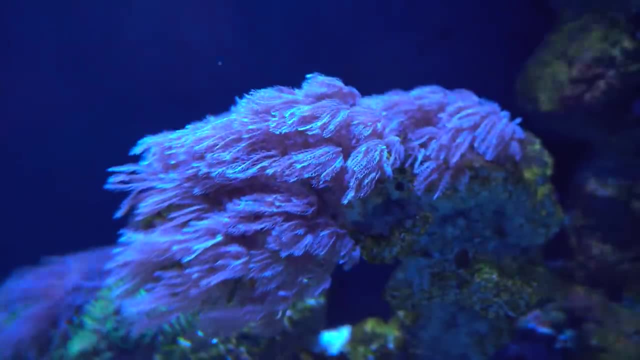 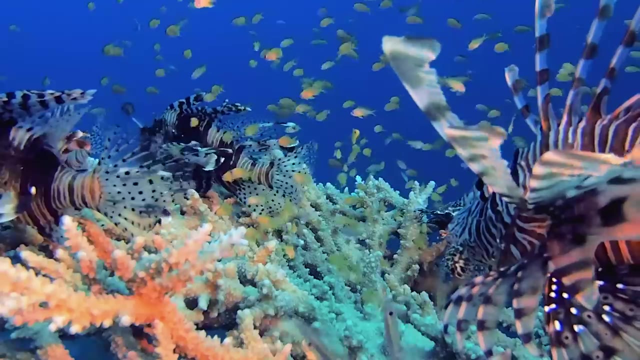 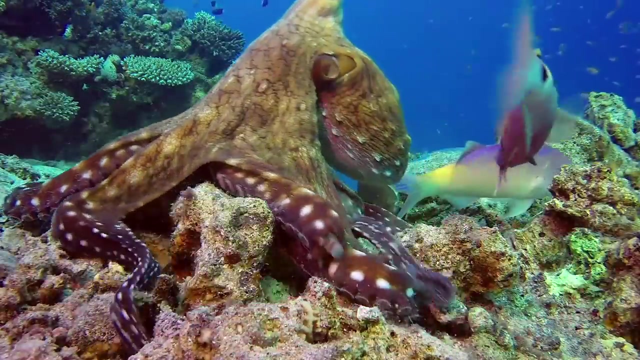 In return, the coral helps the algae to survive. The algae attached to the coral gives coral its beautiful colors. The ocean is the largest habitat for animals in the world. The animals of the ocean either live in the deep open sea or they live on both the land and in the water. 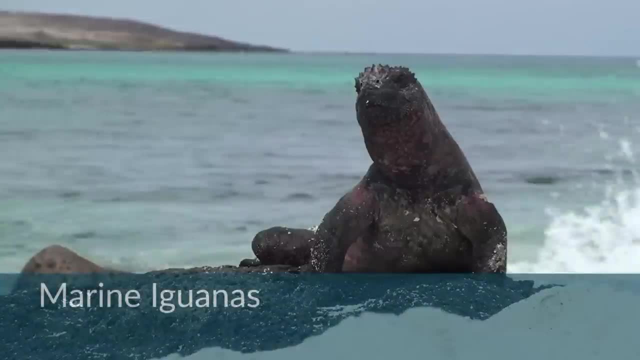 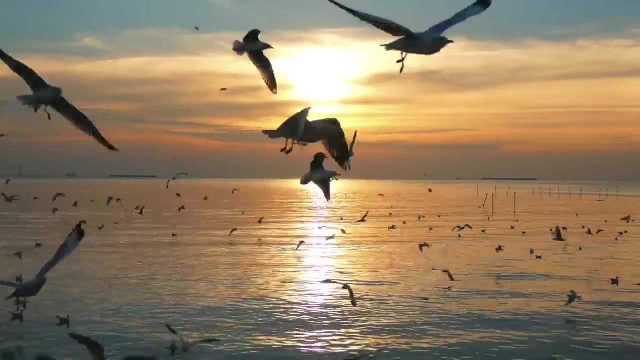 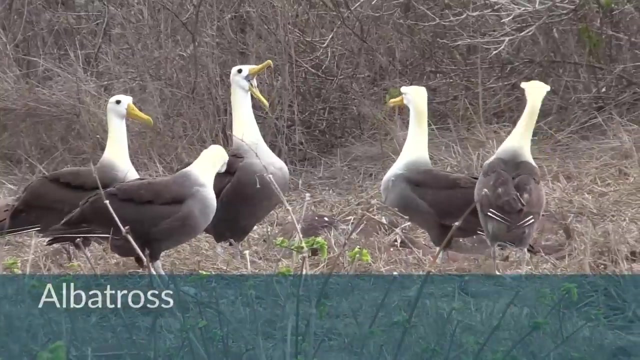 Sea turtles and saltwater crocodiles, marine iguanas and polar bears depend on the ocean for their food. There are also many seabirds that rely on the ocean for survival, including penguins, pelicans, tern, albatross, puffins, gulls and others. 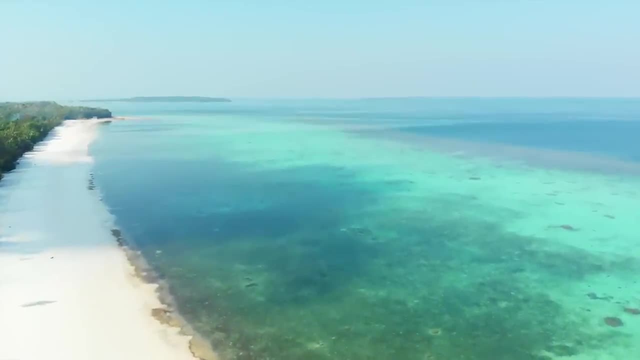 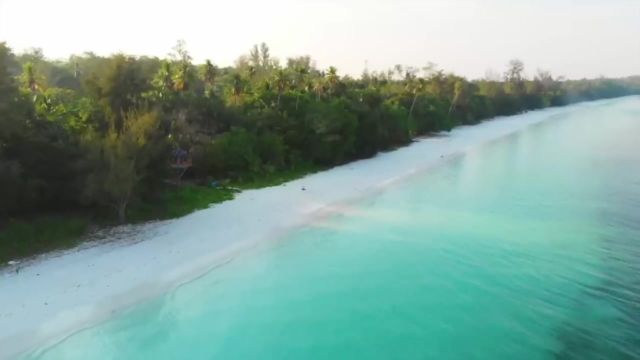 Not all these animals, birds and plants live in or near the same oceans. Some of the oceans are very cold, with parts covered in ice, while others are warm and cold. Some of the oceans are very cold with parts covered in ice, while others are warm and cold with parts covered in ice. 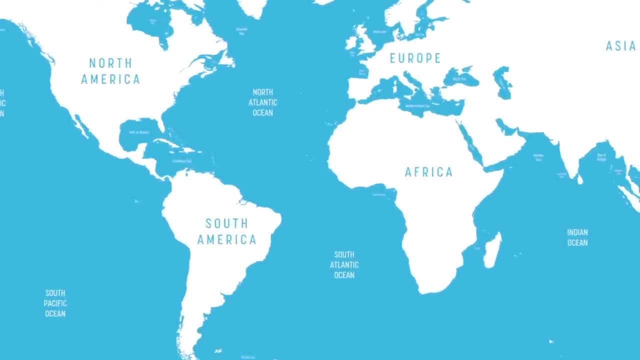 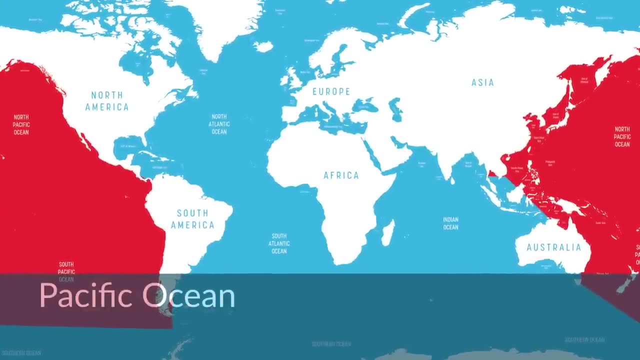 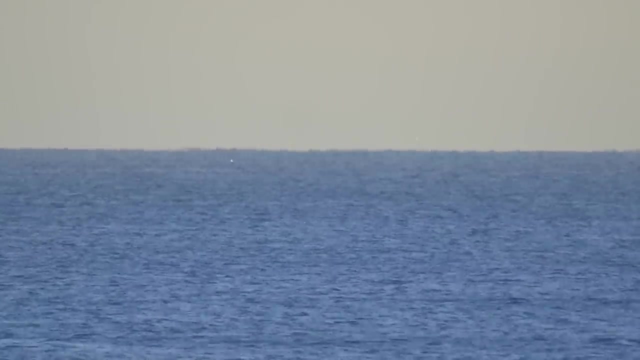 Let's take a closer look at each of the five oceans and see how they're different and similar. The Pacific Ocean is located between North and South America and Asia and Australia. It is the largest ocean in the world. If we combine all the land on Earth, the Pacific Ocean would still be bigger. 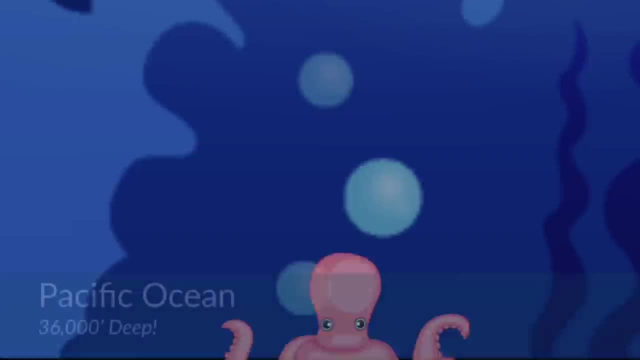 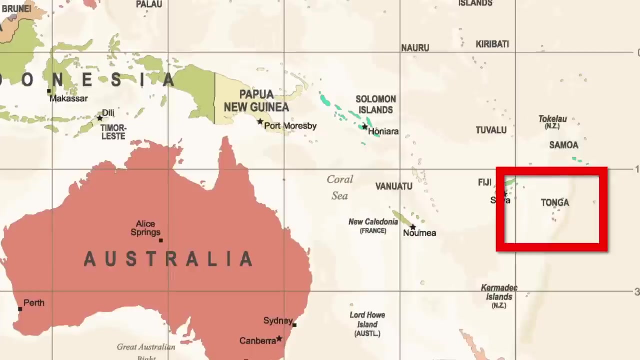 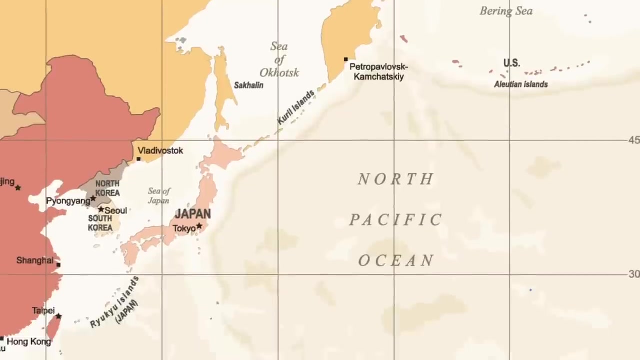 It is also the deepest of all oceans: It is 36,000.. It is 36,000 feet deep. The islands of Hawaii, Samoa, Tonga, Fiji and New Zealand are in the Pacific Ocean. In fact, there are thousands of islands in the Pacific Ocean. 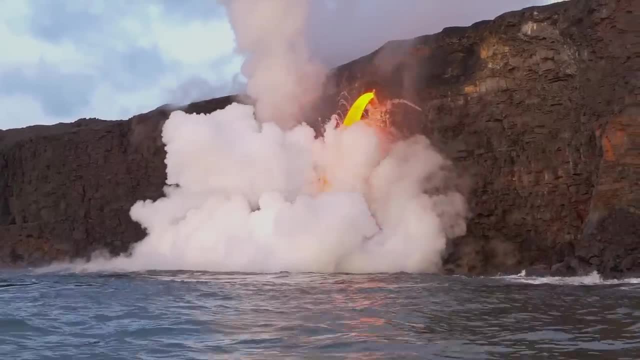 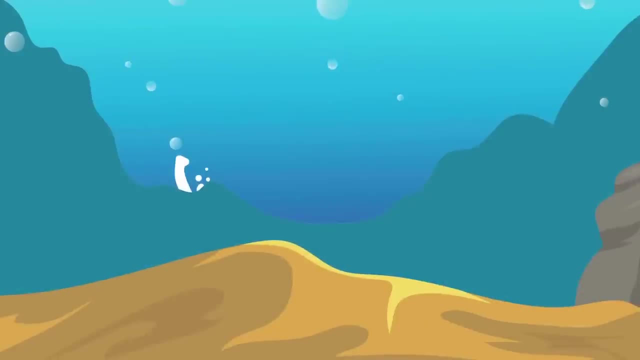 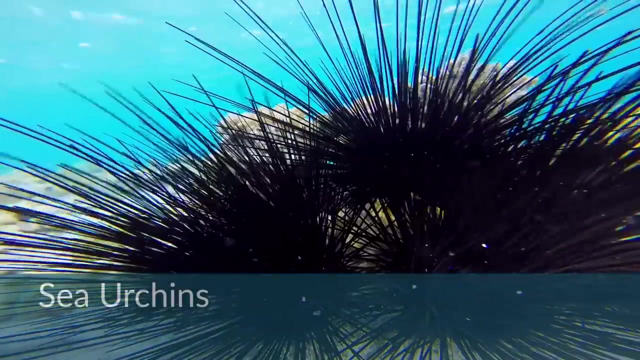 Something cool about the Pacific Ocean is that there is an area of hundreds of active volcanoes under its surface called the Ring of Fire. The plant life in the Pacific Ocean is kelp, Algae, and other sea creatures are also present. seaweeds, as well as seagrass, Sea urchins, snails, abalone and crab also live in the Pacific Ocean. 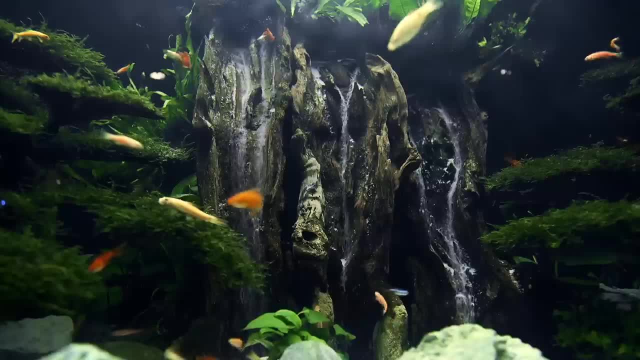 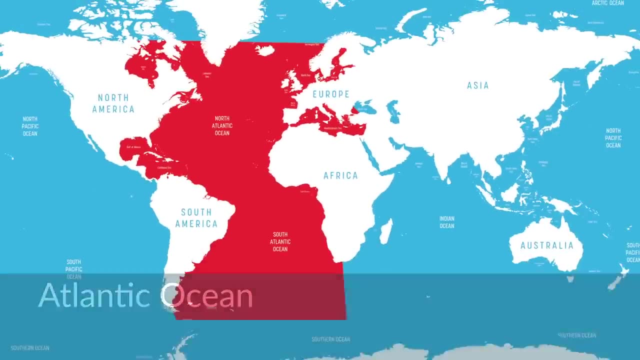 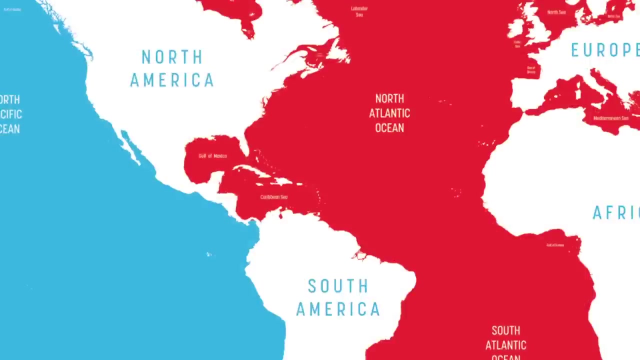 Seaweed gives smaller animals in the ocean a place to live and hide from larger animals and predators. The Atlantic Ocean is the second largest ocean. It is the saltiest of all the oceans. This ocean is between North and South America on one side and Europe and Africa on the. 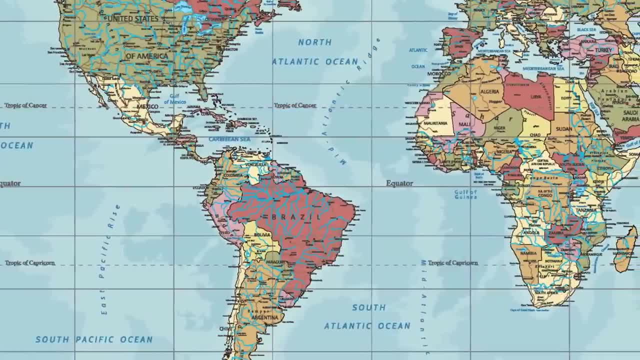 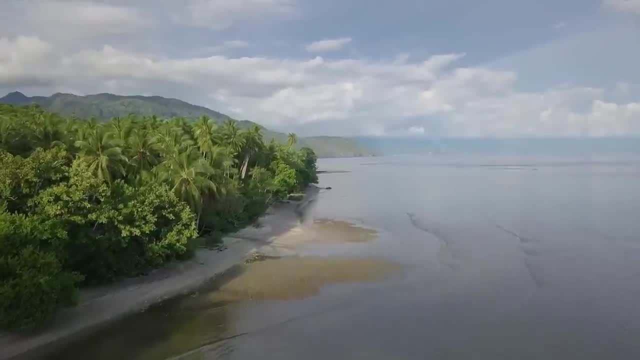 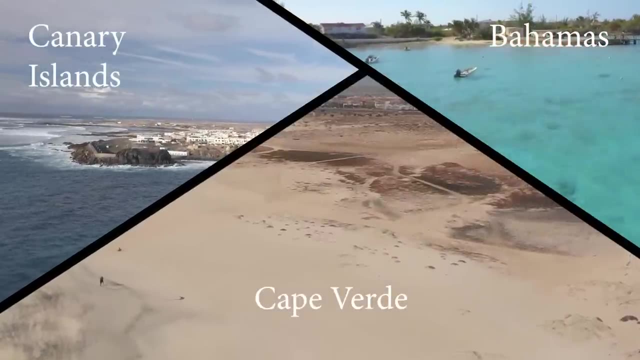 other. The Atlantic Ocean is divided up into North and South Atlantic by the equator that runs through the middle of it. The water that is near the equator is warmer. Cape Verde, Canary Islands and the Bahamas are islands in the Atlantic Ocean. Greenland is also in the Atlantic Ocean. 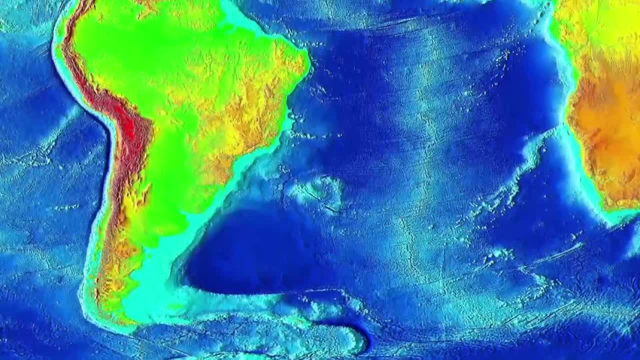 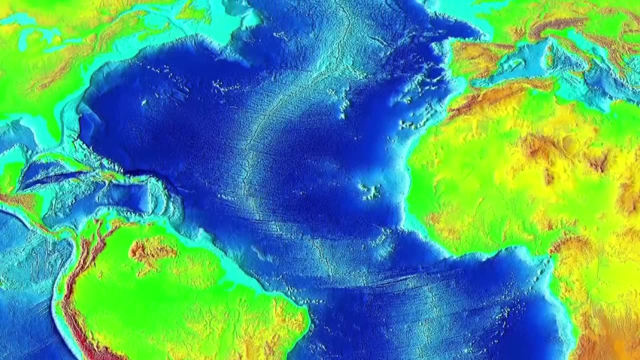 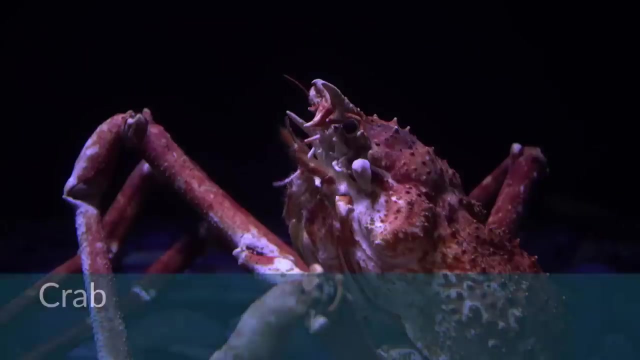 It is the largest of the oceans island on Earth. Something unique about the Atlantic Ocean is that there is mostly an underground mountain range that runs right through it, called the Mid-Atlantic Ridge. Dolphins, sea turtles, clownfish, coral crab and salmon live in the Atlantic Ocean. 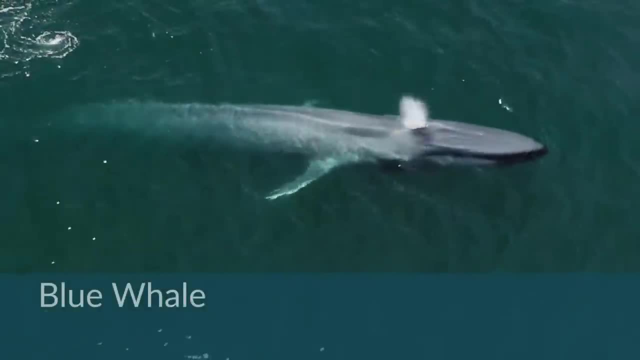 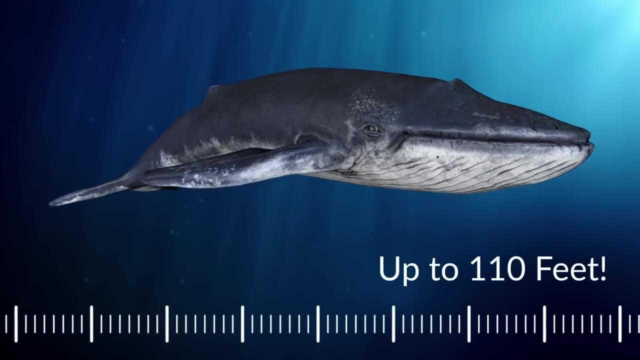 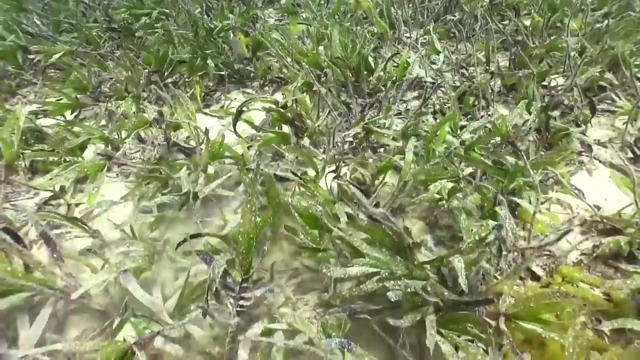 Larger fish like the bull shark and the blue whale also inhabit this ocean. The blue whale lives in saltwater oceans like the Atlantic. It can grow to be 110 feet long. The main plant life in the Atlantic Ocean is algae, seagrass, seaweed and phytoplankton. 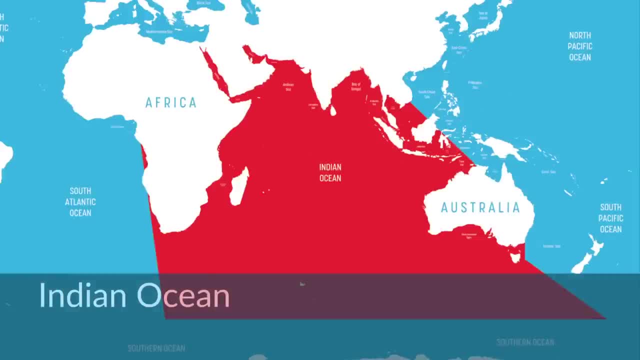 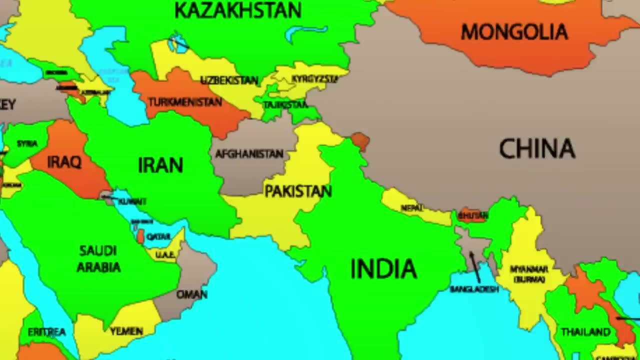 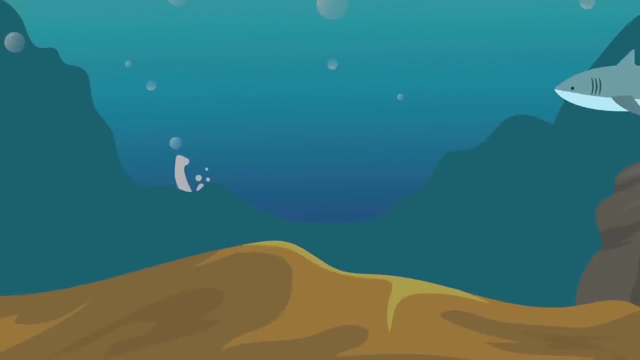 The Indian Ocean is the third largest ocean. The borders of the Indian Ocean are Africa, Australia, Iran, Pakistan and India as well, As well as Antarctica. Some of the marine life found in the Indian Ocean are sharks, whales, dolphins and various 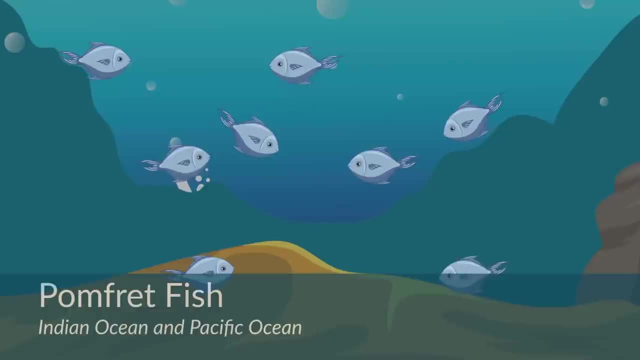 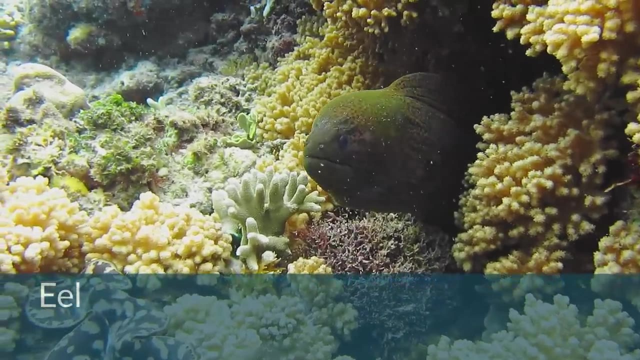 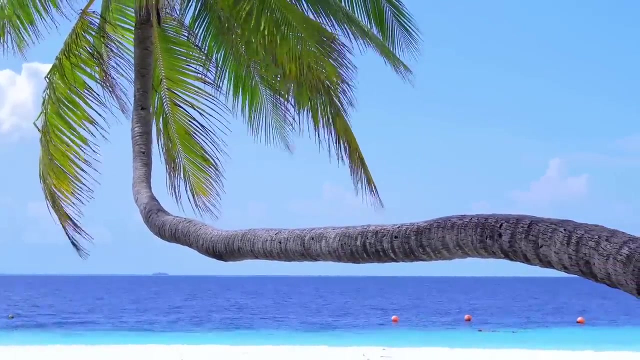 sea turtles. Pomfret fish are found in both the Indian Ocean and the Pacific Ocean. Eels also have been found in this ocean. The Indian Ocean is the warmest ocean of the five, so not as much marine life is found there. 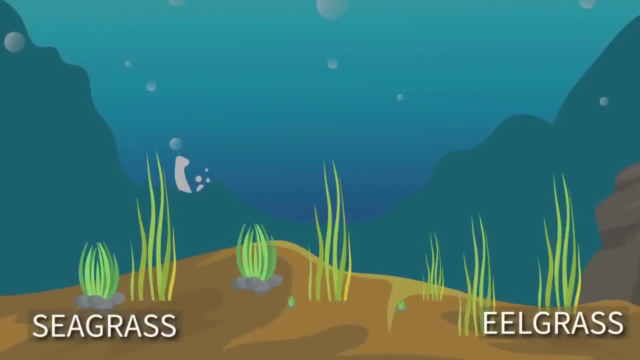 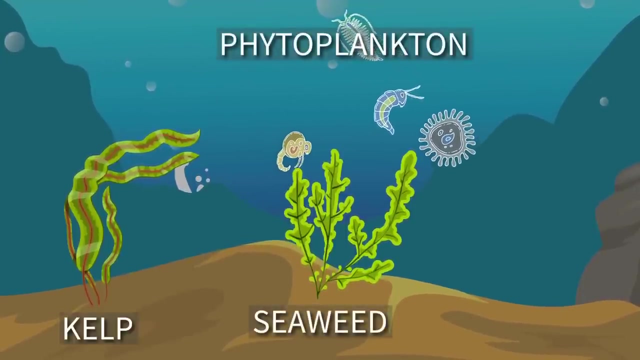 Eelgrass and seagrass are found in the Pacific Ocean. Eels are common plants found in the shallow areas of this ocean. They are the food source for scallops, crabs and many fish. Kelp, seaweed and phytoplankton also live in these waters. 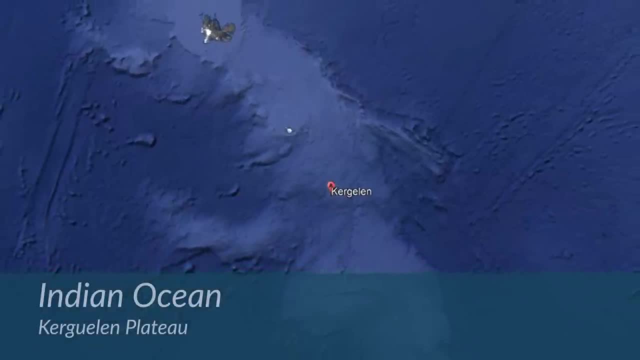 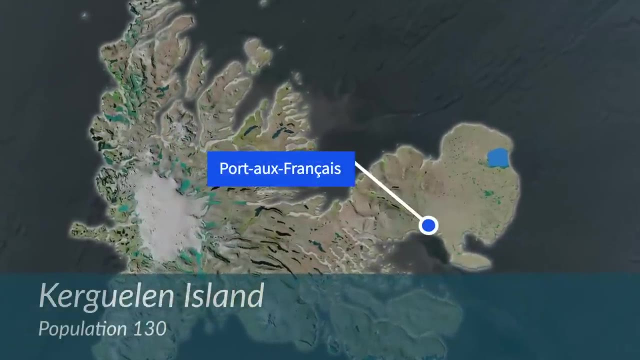 In the Indian Ocean there is a submerged continent formed by volcanic activity named the Kerguelen Plateau. A small portion of it has formed an island that only 130 people live on. The southern part of the island is known as the Kerguelen Plateau. 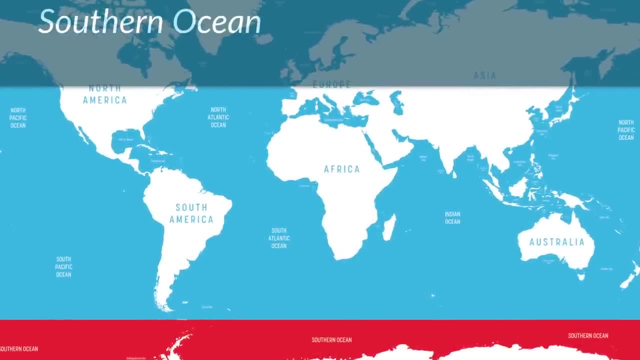 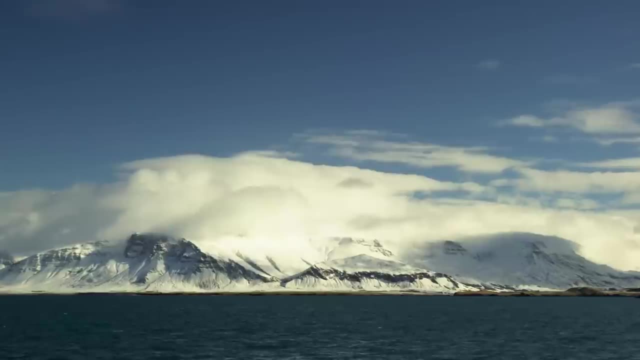 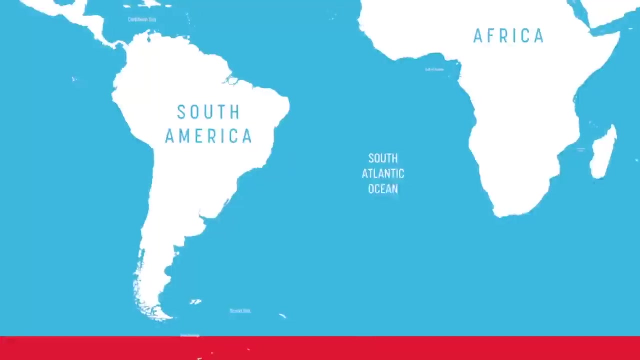 The Kerguelen Plateau is the largest island in the Indian Ocean. The southern ocean is also known as the Antarctic Ocean. This ocean circles Antarctica and is the most southern of all oceans. It is the fourth-largest ocean. Parts of it freeze in winter and then melt again in summer. 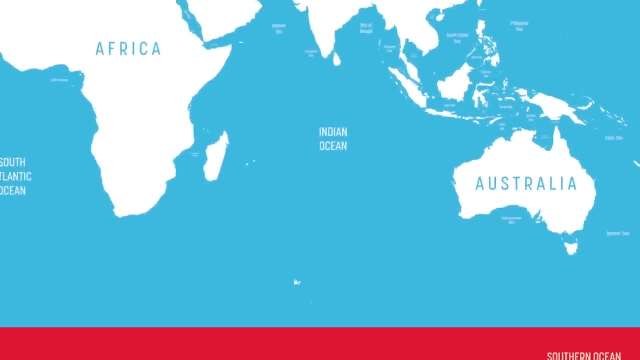 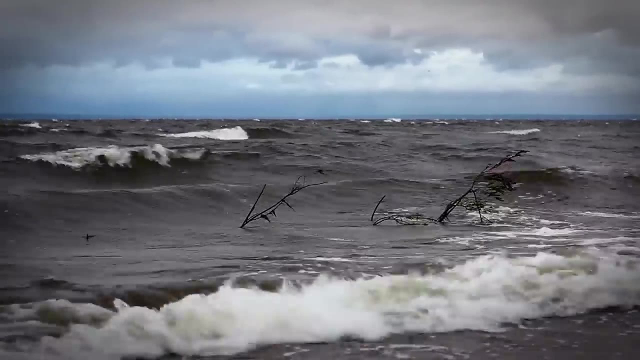 Chile, Argentina and Australia are some of the countries that border the southern ocean. This ocean is known for its stormy waters and can be quite dangerous Because it is so open and wet. the ocean can be very dangerous When it is cold and windy. it creates enormous waves. 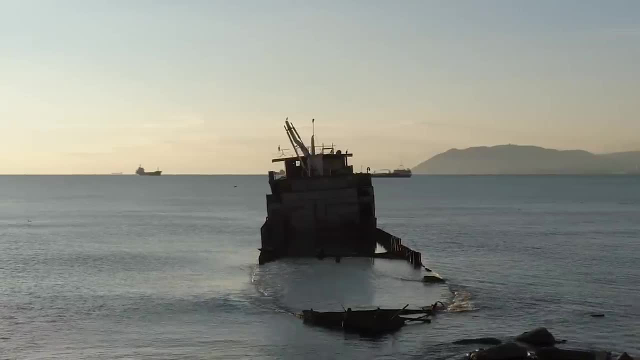 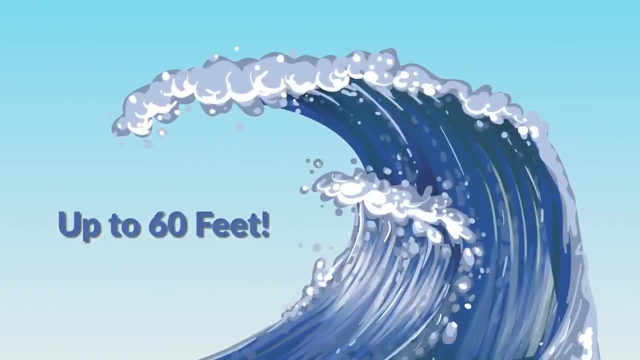 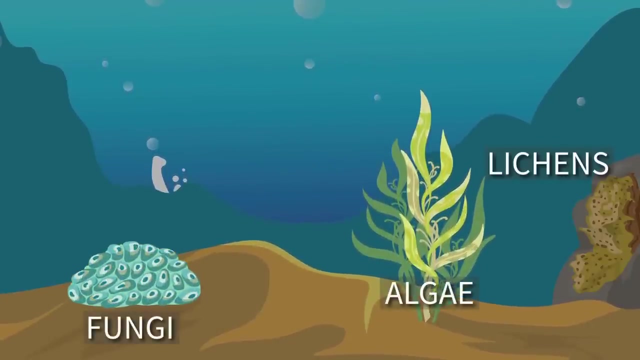 Some over 32 feet high, are very dangerous for ships passing through its freezing waters. Scientists have even discovered waves twice that tall. Fungi and algae are some of the plant life that exist in this ocean. The Arctic Ocean is the smallest, shallowest and coldest of all the oceans. 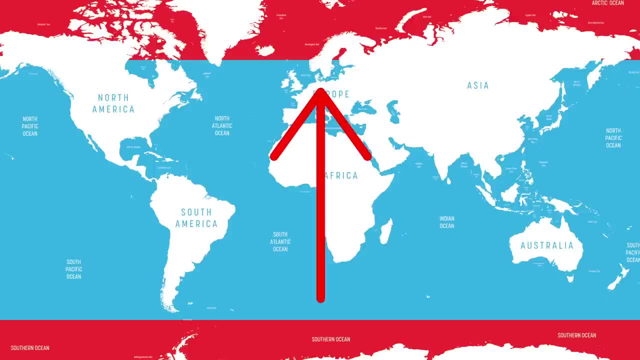 It is on the opposite side of the world from the Pacific Ocean. The Arctic Ocean is the smallest, shallowest and coldest of all the oceans. It is on the opposite side of the world from the Pacific Ocean. Theappy delta, бел morning sun is the northernmost in the Arctic Ocean. 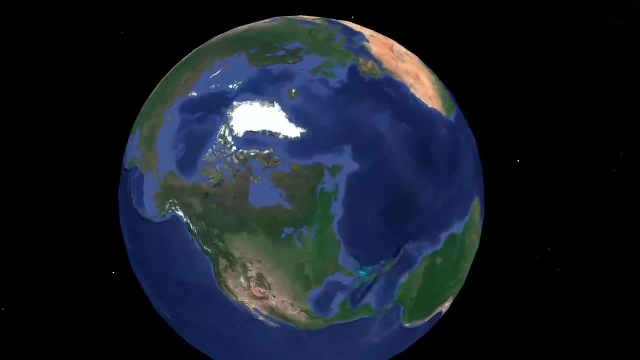 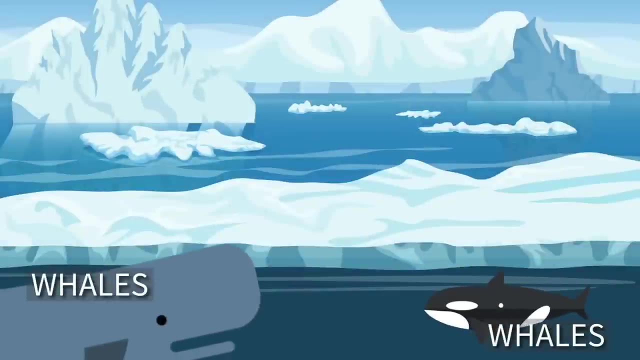 The Arctic Ocean is the lowest most famous flagship environment in the Arctic Ocean. It has the largestладเลย, 174 feet. Then it is a critical living liquid, But 감�ango종이시장окech. 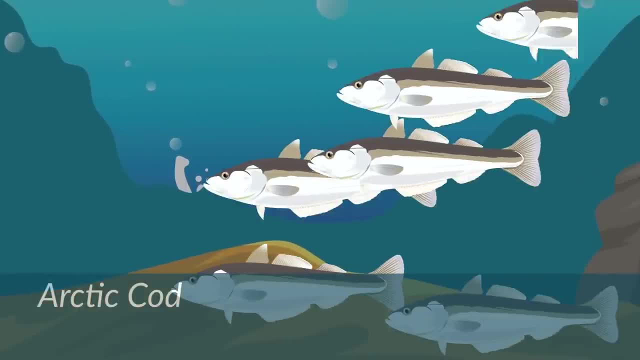 utional unknown 세상. Canada, Asia, Greenland, Europe and Alaska almost surround this ocean entirely. Whales, polar bears, walrus and seals live in and near the ocean. The arctic cod is a fish that lives in the Arctic Ocean. 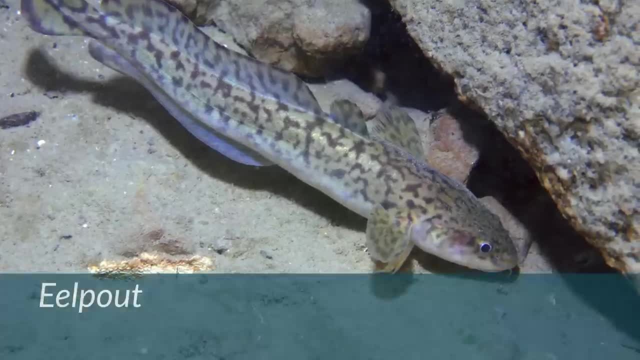 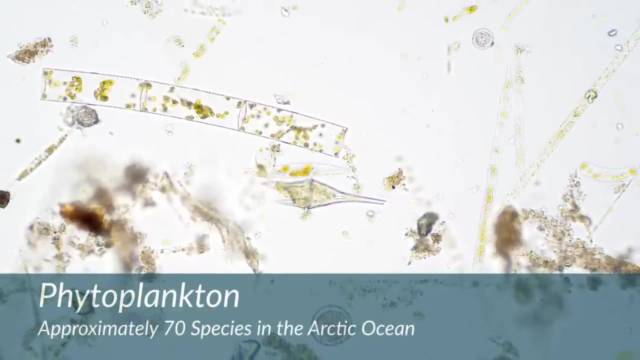 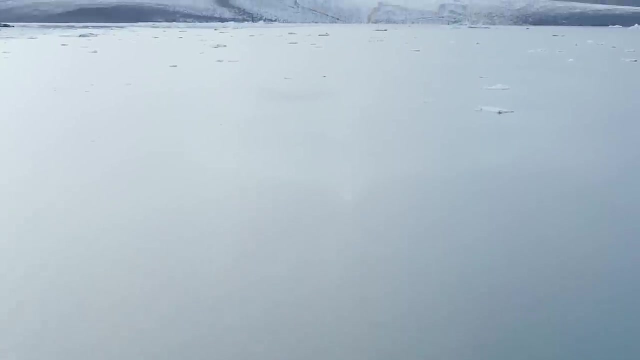 They don't reproduce, strengthen, sometimes In large numbers, as well as snailfishes, ohnezeko, anded Transforming, 70 species of phytoplankton found in the Arctic Ocean, as well as Arctic seaweed and Arctic moss. As you can see, there are many types of plants and animals living in and near the world's oceans. 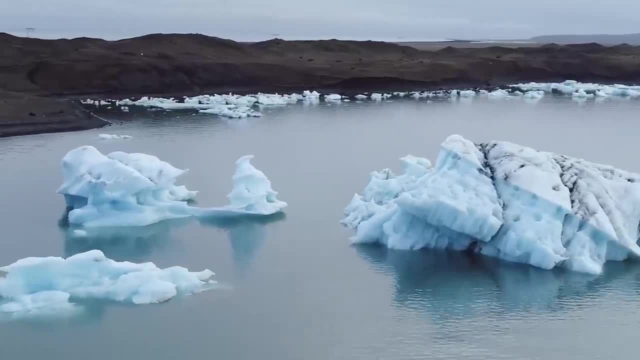 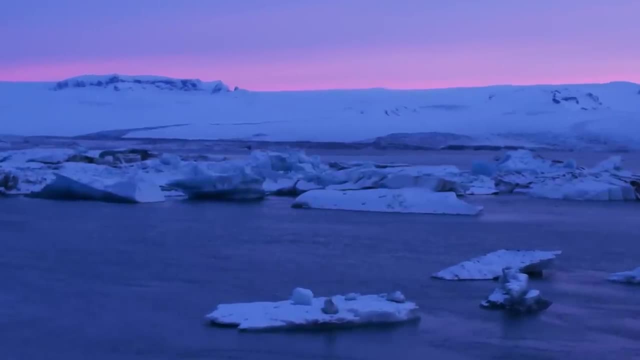 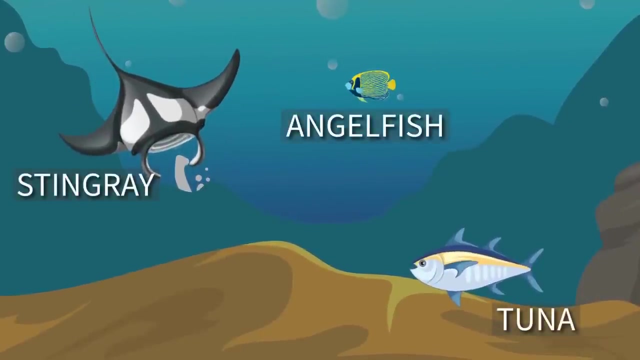 It is a giant habitat where many of the living organisms rely on each other to stay alive. There are many types of fish living in the world's oceans. Here are just a few: Tuna, stingrays, angelfish, clownfish, sardines and cod.